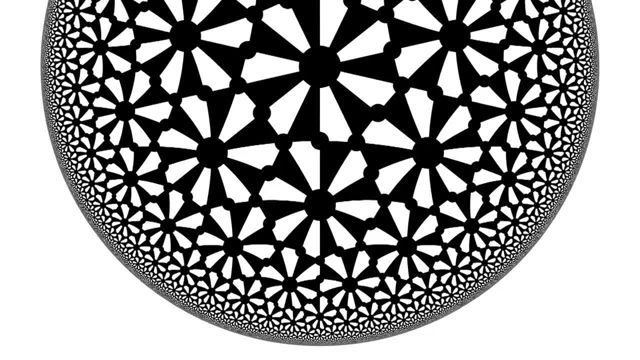 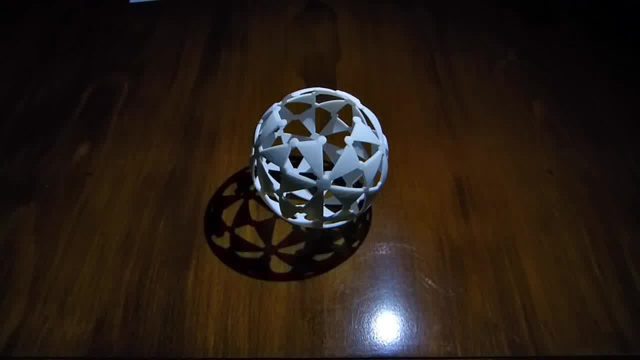 Subtitles by the Amaraorg community. The best known map or model of the hyperbolic plane is the Poincaré disk model. This was first discovered by Beltrami. To understand this model, let's go back to the sphere for a bit. 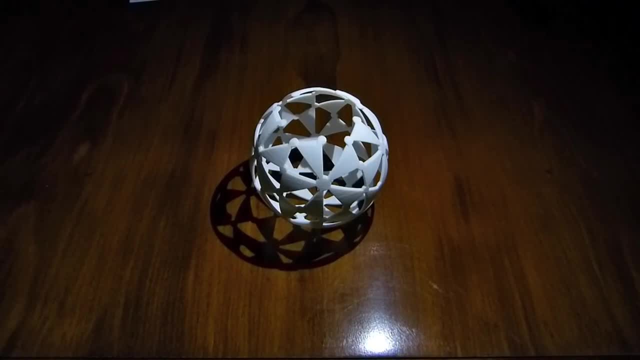 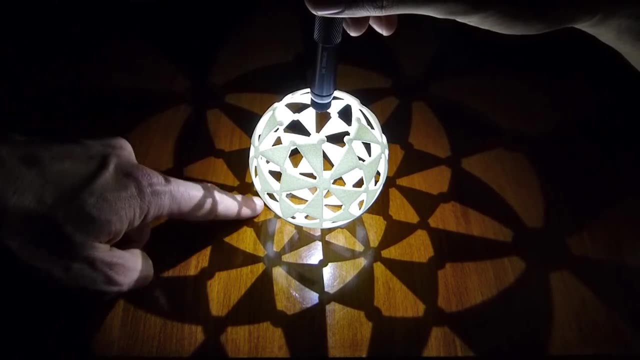 This sphere is 3D printed with a tiling by identical triangles. When we stereographically project the tiling to the Euclidean plane, sizes are distorted. The triangles here look much bigger than the ones here. Let's compare the sphere tiling to a tiling of the hyperbolic plane. We can't see the 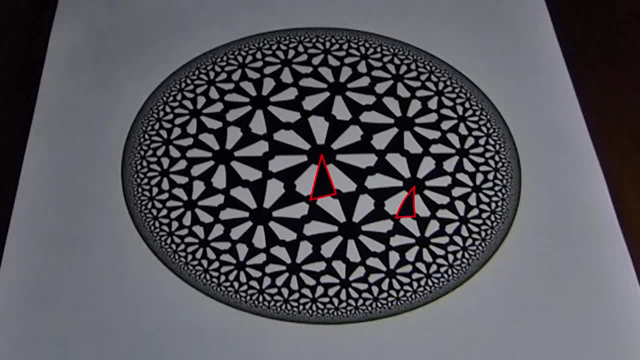 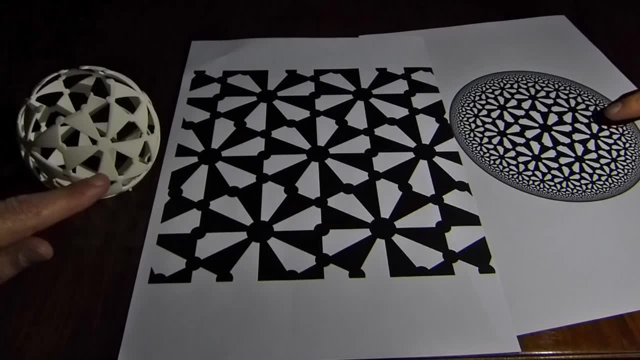 true hyperbolic plane. We can only see the model. All of the triangles are identical, even though they look different in the model. Before we continue, we should really say what a triangle is. It is a figure with three sides, each of which is a geodesic. That is a shortest path between nearby points. 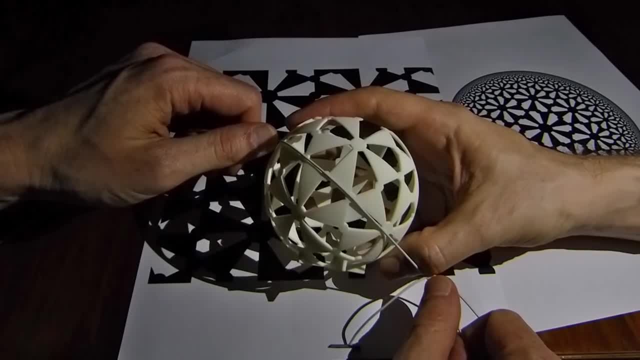 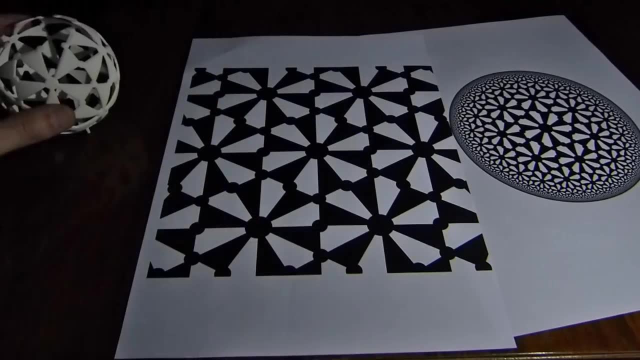 On the sphere. geodesics are great circles. For example, the equator is a great circle. Note that any pair of great circles meet exactly twice In the Euclidean plane. geodesics are ordinary straight lines. Note that now geodesics either. 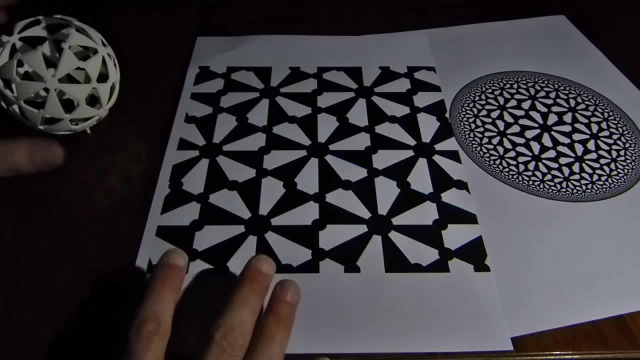 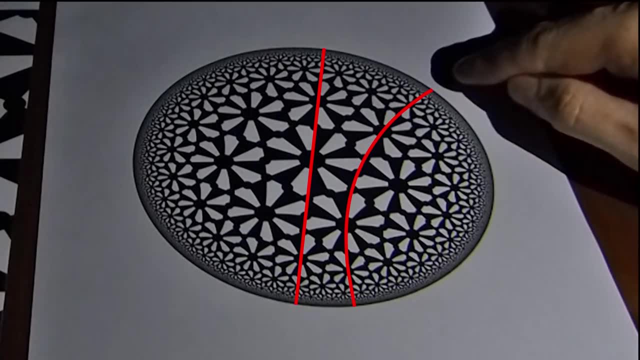 meet once or meet zero times, That is, they are parallel. In the Poincaré disk model, the geodesics are straight lines through the center or arcs of circles that are perpendicular to the boundary of the disk. Here the string doesn't tell us where the geodesics are. Again, this is because we can. 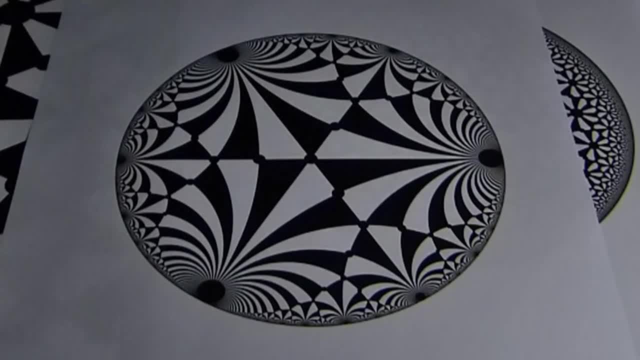 only see the distorted projection, not the true geometry. In the hyperbolic plane, geodesics can only meet once, meet once at the boundary or meet zero times. Although lengths are distorted, angles are still correctly represented. This is just like stereographic projection. This is just like stereographic projection. This 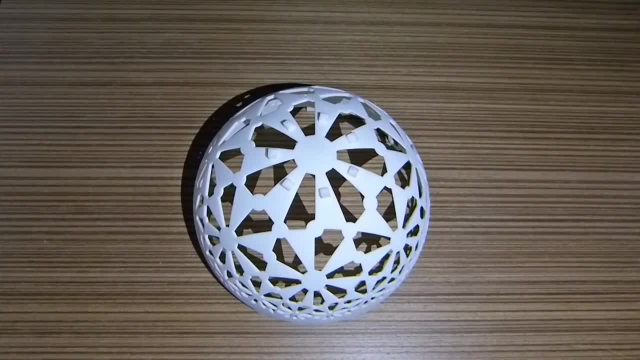 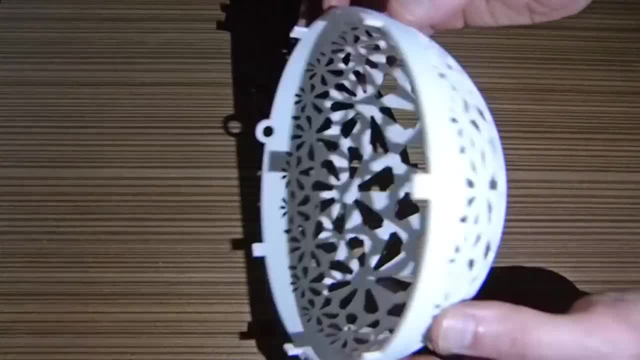 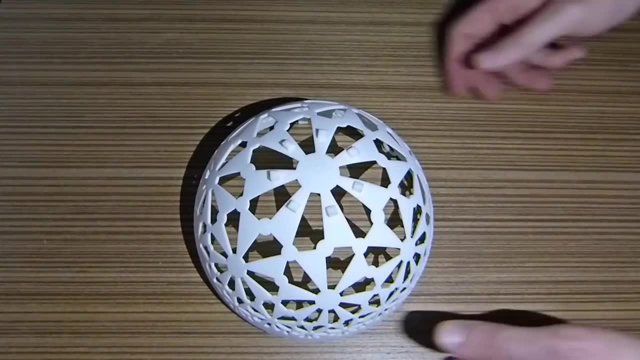 hyperbolic plane inside of Euclidean space. Here is a 3D printed hemisphere model. In this model, geodesics are intersections of the hemisphere with vertical planes giving circles perpendicular to the boundary. Again, lengths are distorted, but angles are correct.